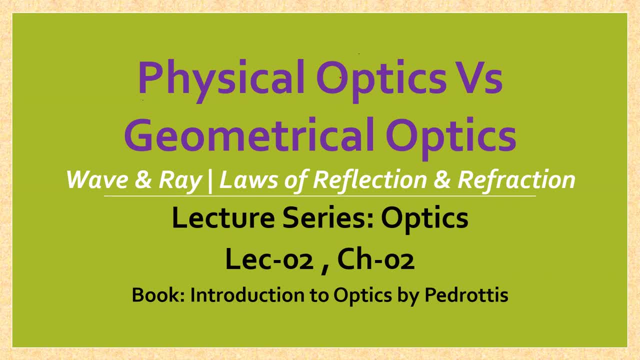 we will discuss laws of reflection and law of reflection Basically in our lecture series. we are following two books. First is our main book, which is Introduction to Optics, by Pedrotti's family, and second is our book which is Physics for Scientists and Engineers by 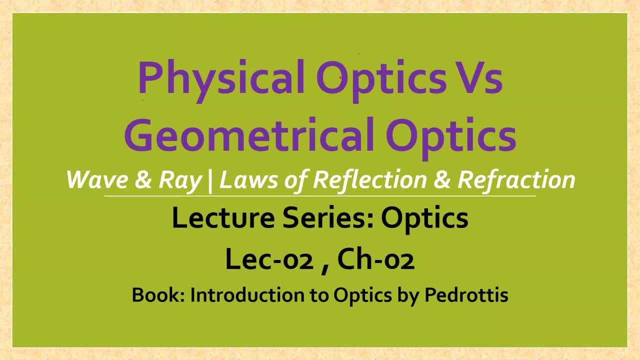 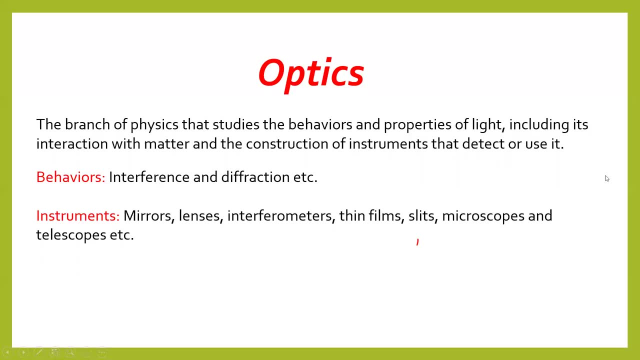 Sarvain Jivit. This is chapter number two of Introduction to Optics and lecture number two. So, students, first of all we will discuss who is optics. We discussed this in lecture number one as well. So optics is basically a branch of physics in which you study light and all the things. 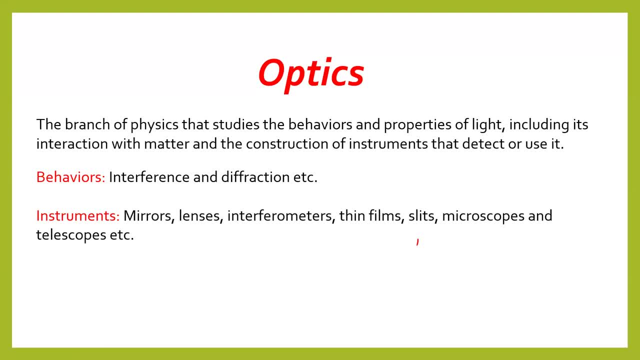 related to light, ie properties of light, behaviors of light or the instruments related to light we use. we study them. So all these come in optics. What is meant by behavior? Behavior is meant by interference, experiments, diffraction, thick and thin films And instruments. 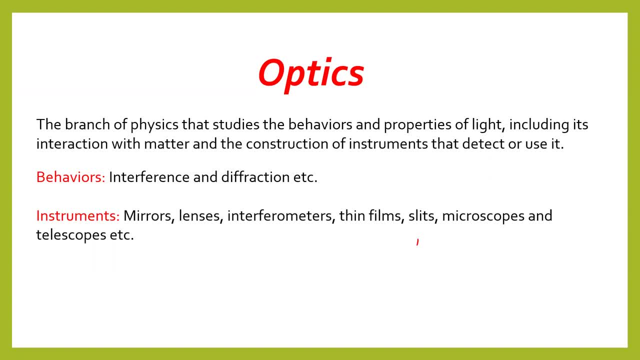 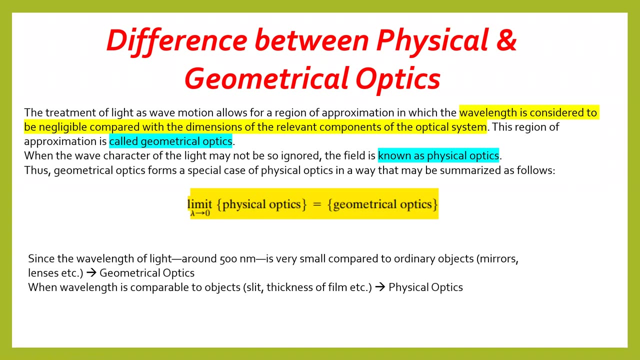 are used in optics, in which you have mirrors, lenses, interferometers, microscopes, telescopes, slits and thin films. So all this study falls in optics. Now, optics is further divided into two categories. The first one is geometrical optics and the second one is physical optics. 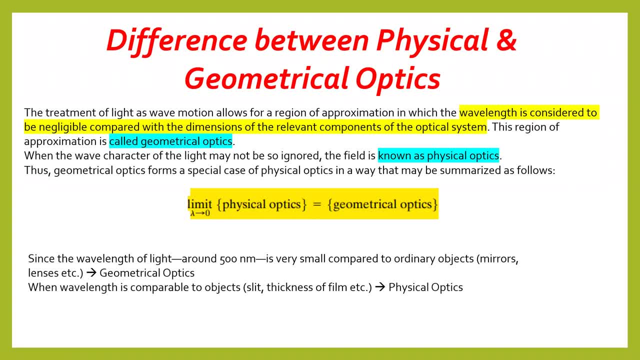 So we usually listen about physical optics and geometrical optics and we should know about the difference between these two. First of all, the main branch. you can say that it is physical optics. In physical optics you consider the wave behavior of light and in all your studies you treat light as a wave. 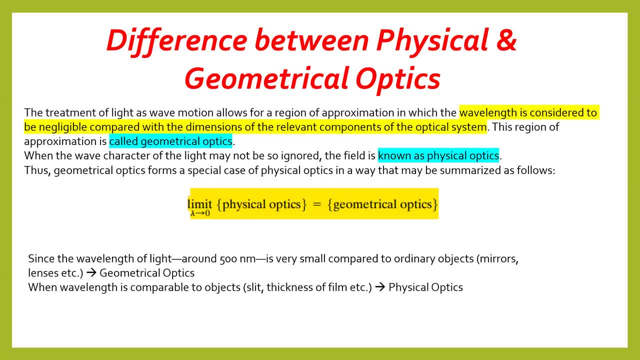 What does it mean to treat light as a wave? You consider the wavelength of light, you study the momentum of light, the wavelength, momentum, energy frequency. you study all these things, you consider them in your study. so you call such a study physical optics. 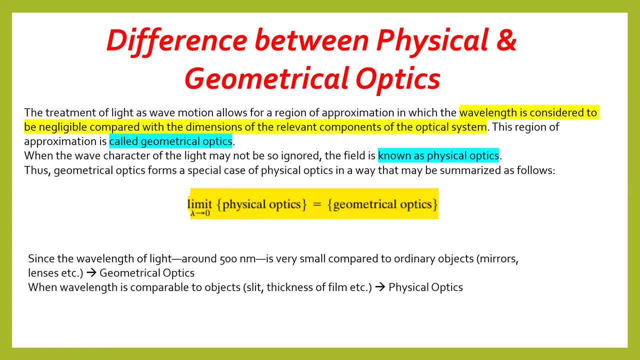 But we have some such experiments or some such phenomena in which we do not have to treat light as a wave. rather, if we treat light as a ray easily, then we can reach our study completely, the actual results. And when you neglect the wave behavior of light or ignore it, 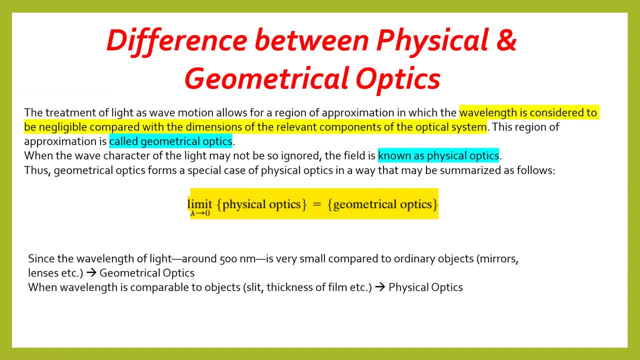 then you call it geometrical optics. okay, So here if I summarize, that when you treat light as a wave, then that is physical optics, And when you ignore the wave behavior of light and consider light as a ray, then that is known as geometrical optics. 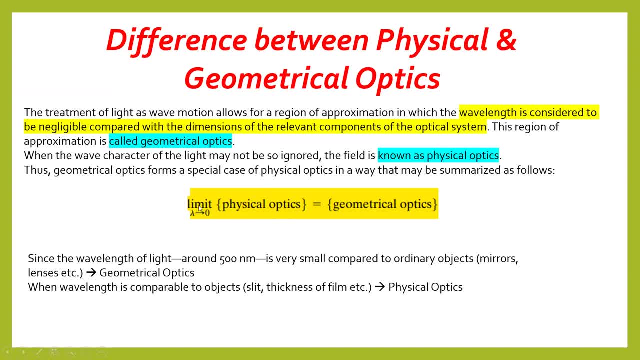 Here I have shown an equation that when you ignore the wavelength, which means limit lambda approaches to zero, then physical optics, the wavelength of light tender to 0.. Sch. Mögliche, Civic, Schematic, Schematic, Schemark, Schnak, Spektak. 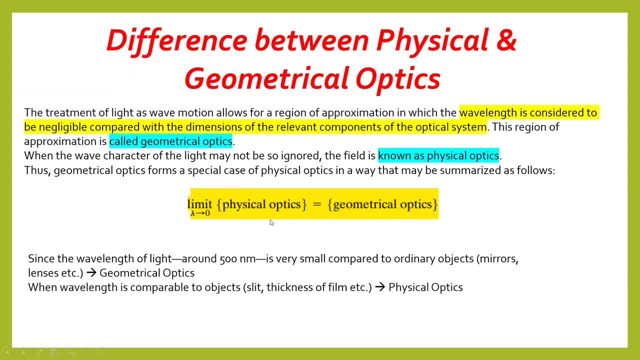 Eigbar Schacaks, Physical, have a special case in which you wanna neglect the wave behavior In the screen. We look at this thing as well. If you consider the wavelength of light, then the wavelength of ordinary light- actually you have, It is very close to five hundred nanometers. five hundred nanometers. 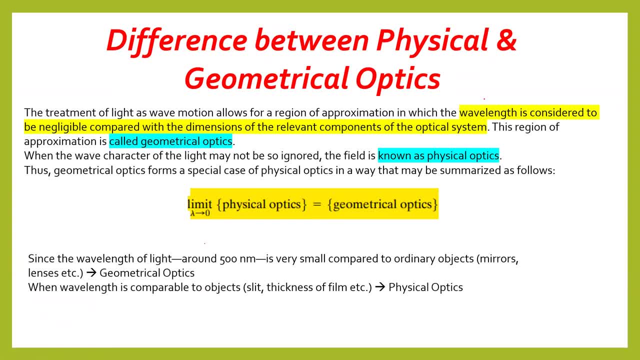 It means that that at Usually the electromagnetic visible spectrum that we have, if you look at it here, then from approximately 350 nanometers to 770 or 780 nanometers, you have visible light. So we are taking its average, that is, approximately 500 nanometers is the wavelength of visible light that you have. 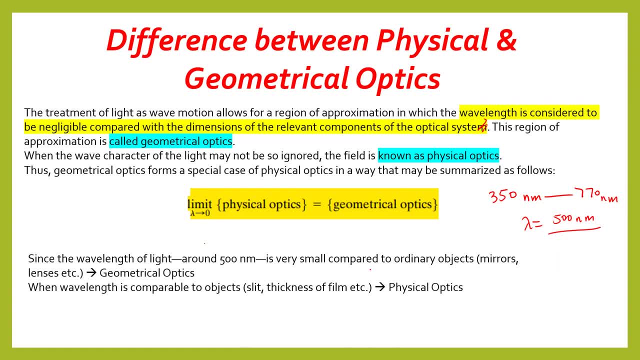 If you consider this length, that is, 500 nanometers, then this length is much smaller than the size of ordinary objects. That is, in the case of mirrors and lenses, this wavelength is much smaller than their size, So that's why we ignore this wavelength and call this study geometrical optics. 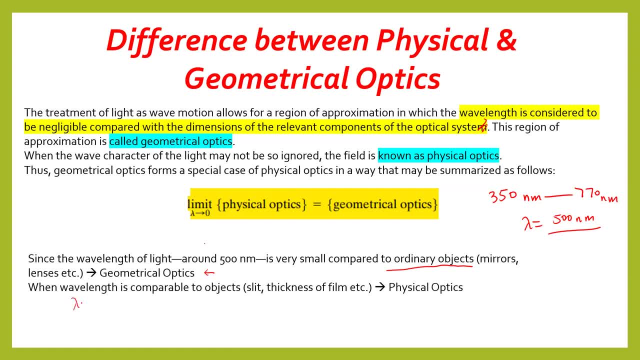 But when you have the size of this wavelength, that is, when you have a lambda of approximately 500 nanometers, then you cannot ignore it. but this size should be comparable or equal to the size of the object And the size of the object. here we have which object. 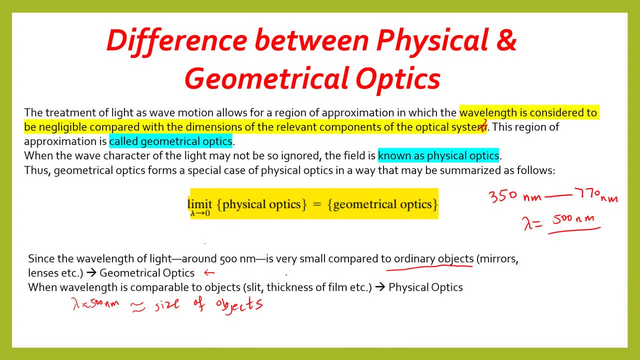 We can have slits. we can have the thickness of the film The way you have thin films. their size can also be in nanometers. The size of the slit can also be very small. So when this size is comparable to each other, then that study is known as physical optics. 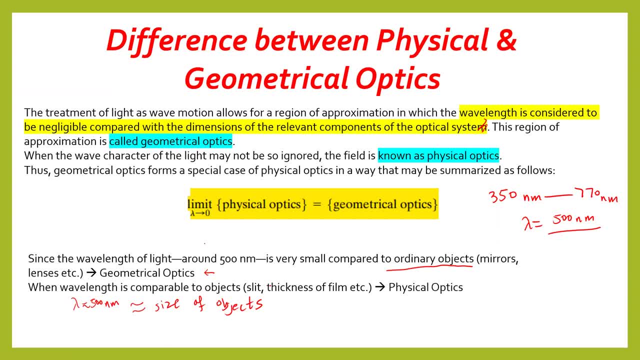 And in that you consider the wave characteristics of light And that is, crust trough, wavelength, momentum, energy. you consider all these things And this study is called physical optics. Next we have let's see The difference between wave and ray. 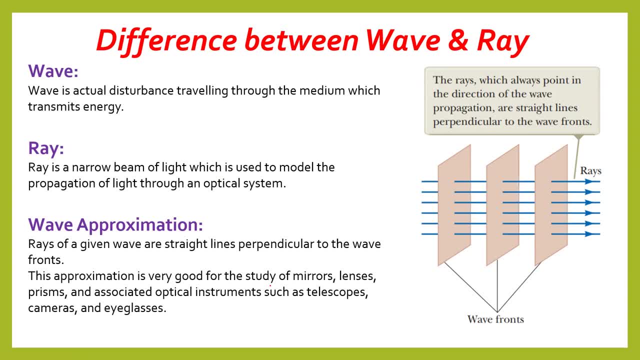 Wave, which is basically- you call it- actual disturbance, which is travelling through the medium. And whenever disturbance travels through a medium, it transmits energy from one point to another point. So when you are considering the wave, you consider the crust trough, wave's crust and trough. 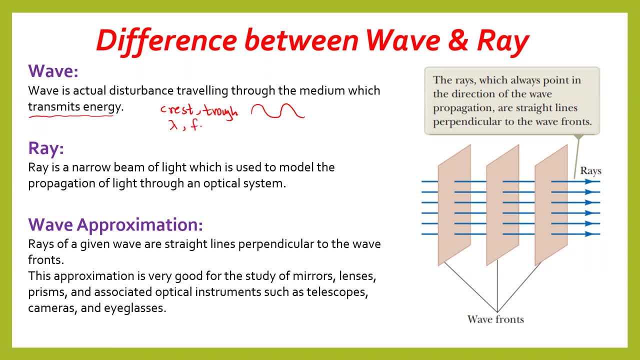 When you will have this behavior of the wave, you will consider the wavelength, You will consider the frequency, You will consider its energy, its momentum, You will be dealing with all these things. So you will have this wave, But you say that the direction in which your wave is travelling, you are just considering that direction. 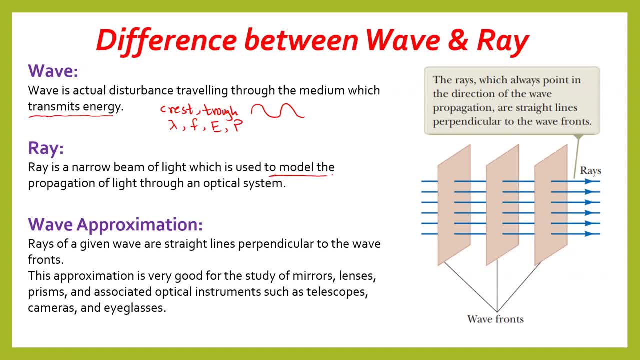 That is, you use the ray to model the propagation of light, That the light or the wave is travelling in which direction. So if you have this wave which is travelling in the right direction, then you can make a ray corresponding to it. 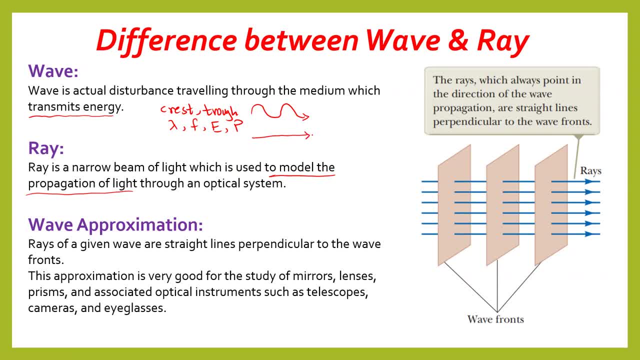 In this way in the right direction. That is, the ray will only tell you the direction of propagation of the wave. So the ray is basically the approximation, And here we see the wave approximation. The wave approximation is that in this approximation you are only considering the direction of propagation of the wave. 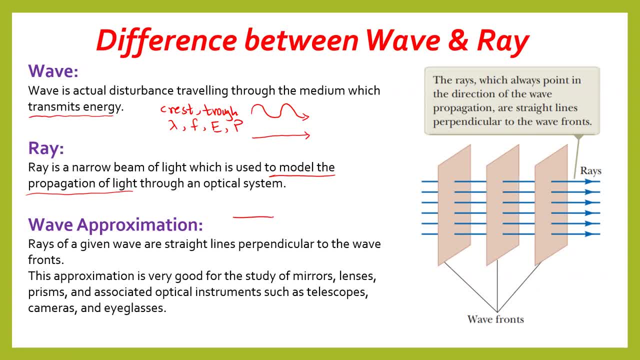 And the direction of propagation of the light is always in the form of straight lines. It is not possible that it is going to bend in this way. Rather, it will always be straight lines and will be perpendicular to the wave fronts. What does the wave front mean? 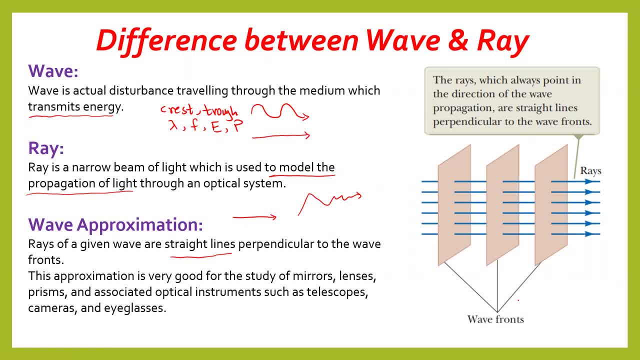 We will study this in detail in the next lecture. Basically, wave fronts can be understood as a sheet And the ray will always be perpendicular to this sheet, As mentioned in the picture here. So this is the meaning of wave approximation. In wave approximation, you are just considering its direction. 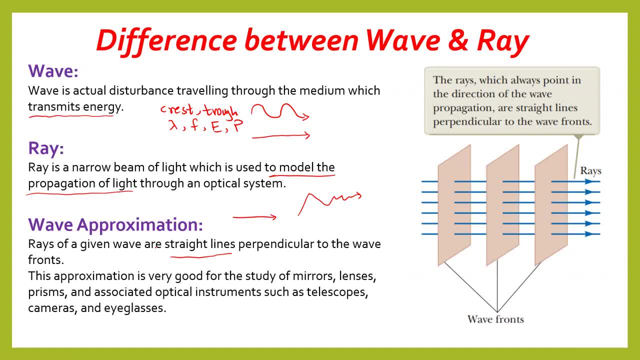 And you are considering that direction in the form of straight lines And you call those straight lines rays. And this wave approximation helps us When we are studying experiments associated with mirrors or lenses or prisms, then we have to consider the direction of propagation of light. 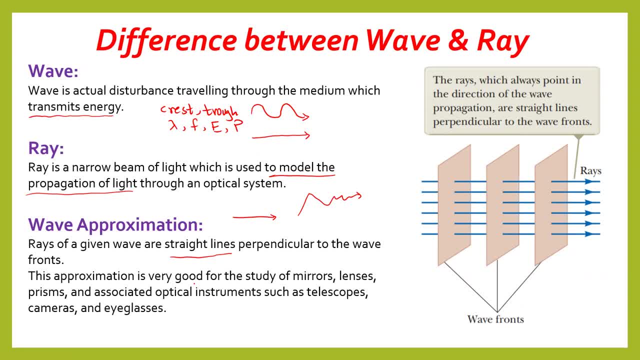 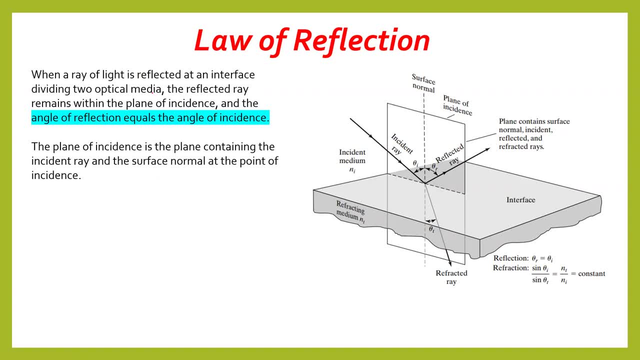 And we model it as a ray. So this approximation is very helpful for us. Now, law of reflection. Law of reflection, We also have it in high school physics. The law of reflection is that if you focus on this figure, So let's say you have medium 1.. 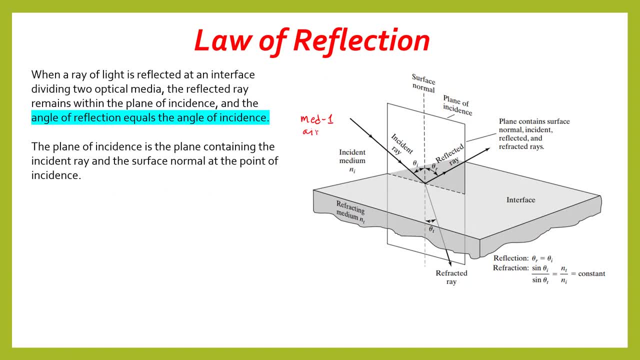 This is medium number 1. You can consider it as air And after that you have medium number 2. Consider it as any slab. You have any material. You can have this medium made of any material. So this is medium number 2.. 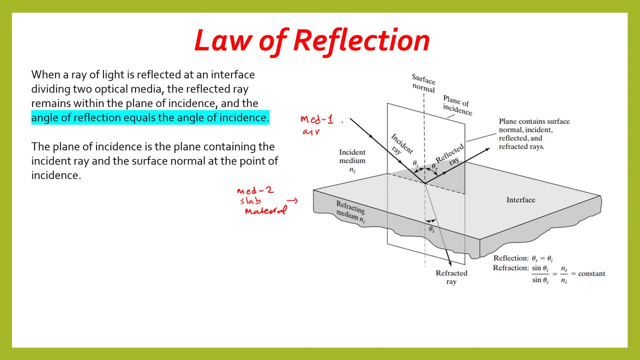 So there is a difference in the nature of both mediums. So when light ray is coming from medium 1, as it has been shown here as an incident ray, This is an incident ray, So it will come while traveling, At some point when it will collide with another medium. 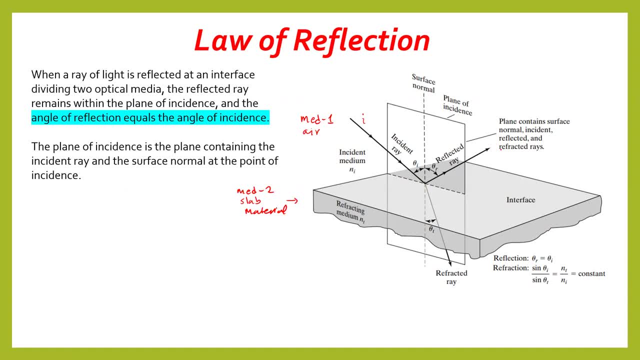 it will bounce back, That is, it will reflect back And the light that will bounce back you call it reflected ray And the coming light is called incident ray. So these rays, both incident ray and reflected ray, always have equal angles with the normal direction. 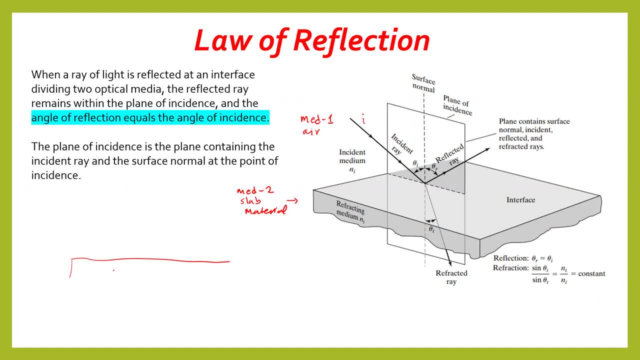 What does normal direction mean? If you had a plane of another medium, then its perpendicular direction- as we have made a perpendicular direction here, which is made with the 90-angle plane, then you call it normal to the surface. Why? Because it is the normal direction of this surface. 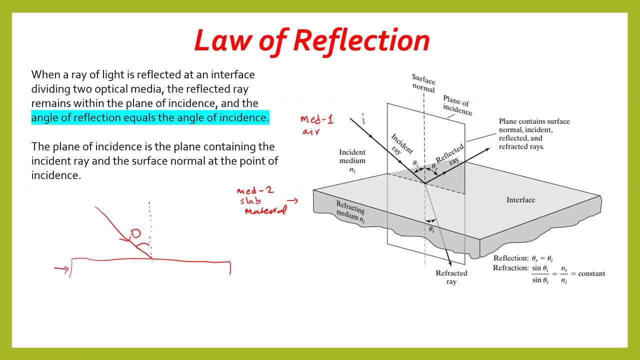 And the incident ray that will come, that angle, theta- i call it incident angle. And when it will bounce back, then the new angle that will be made, you call it theta, reflection or reflected angle. So theta i and theta r will always be equal to each other. 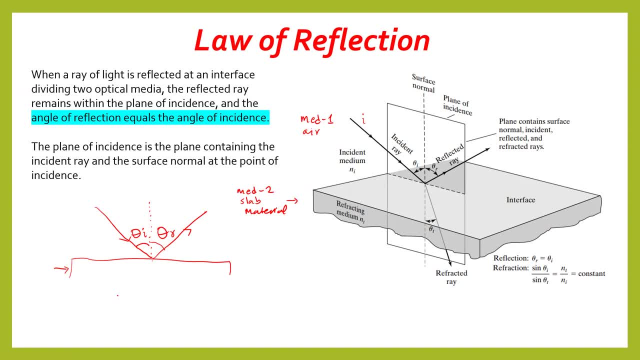 This is called law of reflection, So this has been proved by empirical law experiments. So theta i equals to theta r. This is known as law of reflection. There is one more important thing here, And that is that incident ray and reflected ray 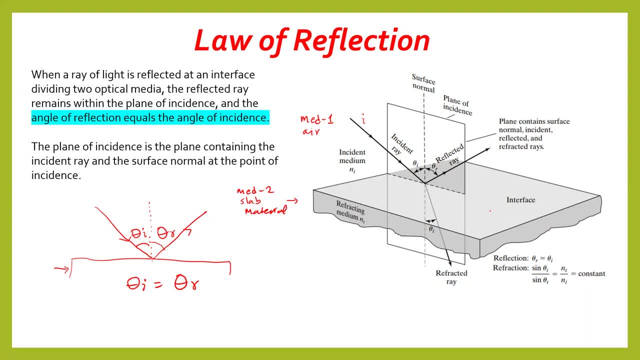 will always be in the same plane, That is, if you have this surface, which is the surface of the second medium, boundary or interface, if you keep a page or a sheet of this, which is 90-angle, which is making the angle of 90 with this second medium. 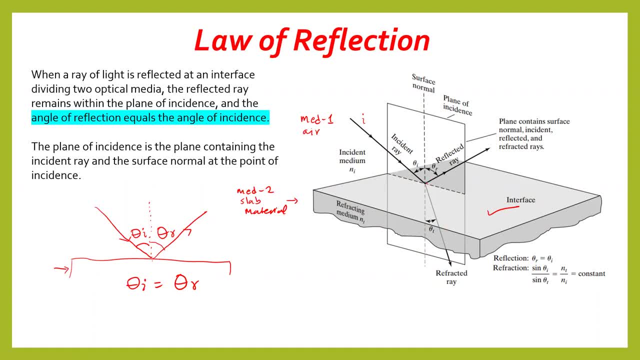 then if the incident ray is coming in the same sheet, then when it will reflect then it will also be in the same sheet, that is, it will lie in the same plane: Incident ray and reflected ray. similarly later in the next topic. 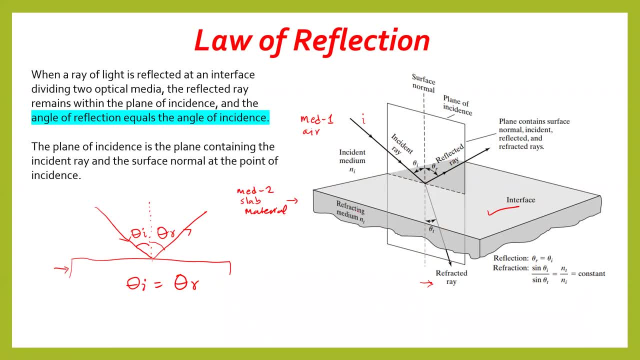 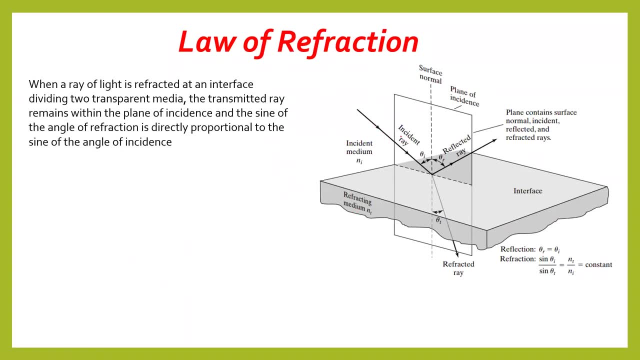 we will see that the reflected ray also lies in the same plane. All three planes are the same. Next is law of reflection. Now, in this, in law of reflection, not reflected ray, but reflected ray- we will study the reflected ray. 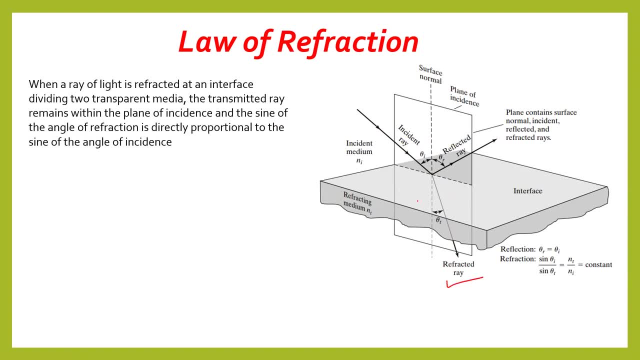 which will travel inside that medium, that is, this ray. So incident ray again you consider, which is traveling in medium 1, it will come and hit at some point. it will hit medium 2, which is its boundary interface. 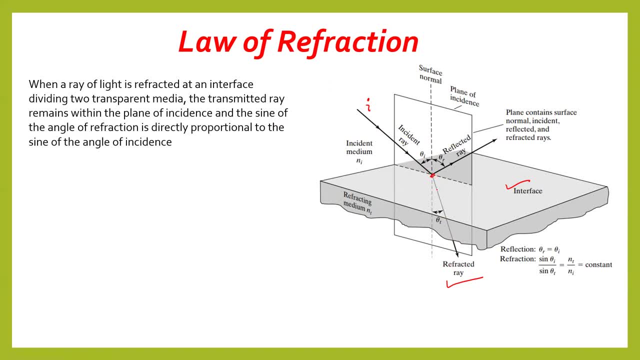 it will come and hit here at this point and then some part of the ray, that is, some part of the light, will travel inside the medium, like light travels inside glass- and some part will bounce back again, The part that will bounce back. 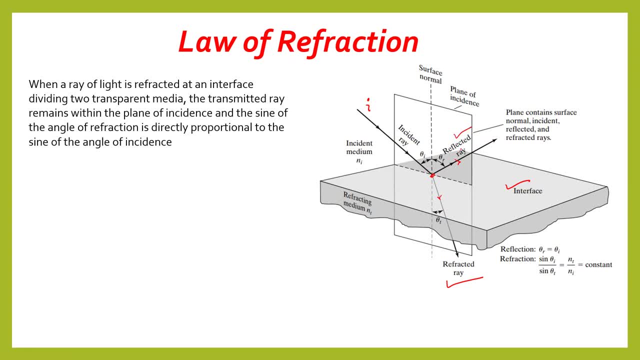 is called reflected ray and we have seen the law of reflection about it And now we are starting to see that the part that will travel inside the medium, the part that will travel inside the second medium of light, about that, the reflected part and the incident part. 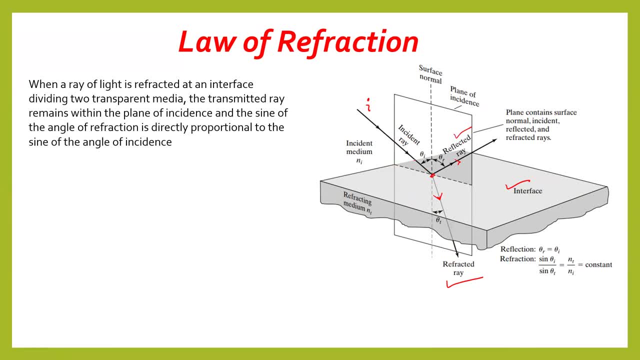 what is the relation between them? So let's say the angle of the incident ray is again equal to theta i, and let me highlight this: this angle is equal to theta i of the incident ray and the light that is reflected. 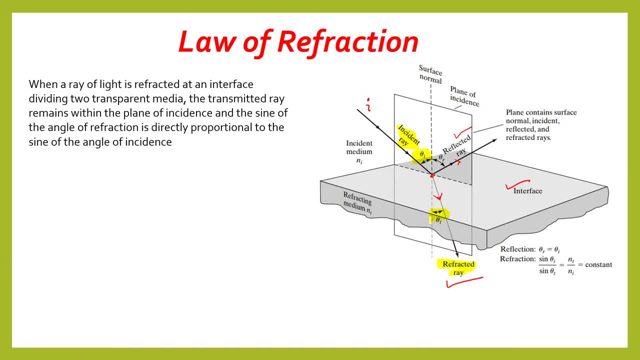 and traveling inside the medium. the reflected ray which you are saying its angle is, let's say, equal to theta t t is said to be that you can also call it transmitted ray, which is transmitted inside the medium. 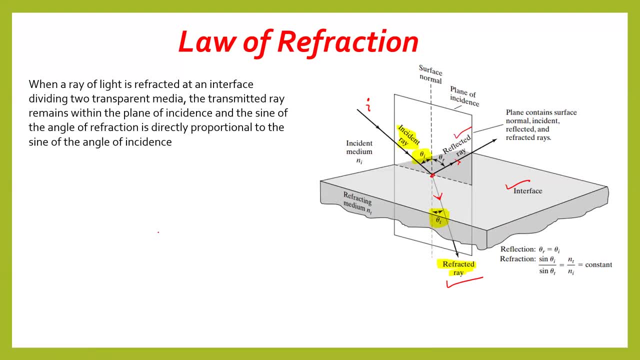 so t basically shows the transmission. So now we have to see what is the relation between them. and that relation tells us law of reflection that incidents, the sign of angle of incidence and the sign of angle of reflection is always proportional to each other. 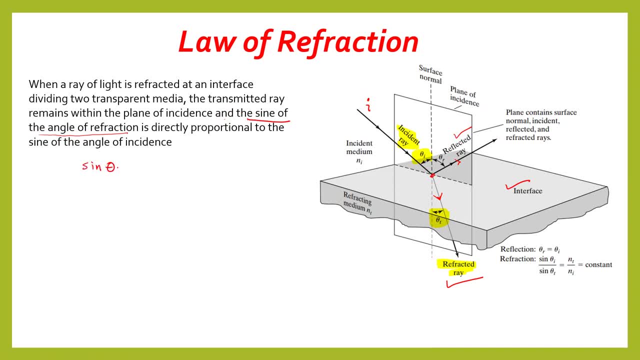 directly proportional to each other, which means sine theta i, that is, the incident angle. its sign is directly proportional sine of transmitted angle. so we have law of refraction. now let's solve this and take it to the complete form. 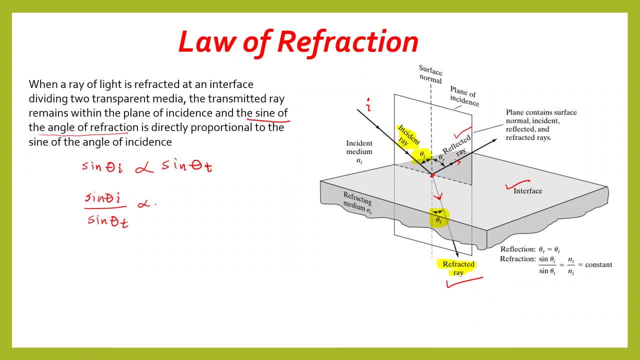 so sine theta i divided by sine theta t, you will have directly proportional to 1k. and when you replace the proportionality sign with the sign of equality, then you will have some constant k. let's say: 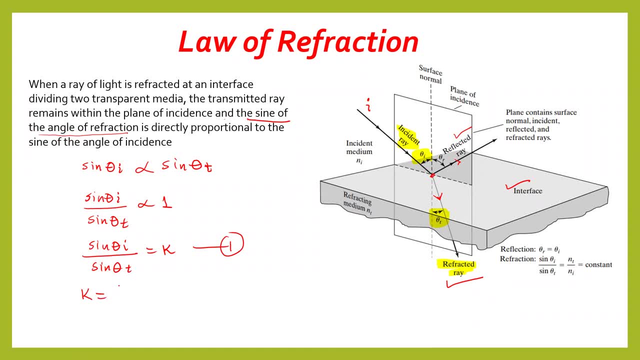 this is equation number 1, this constant, the empirical value of this constant, which is taken out of the experiment. that value is: you have n t divided by n i you put this, which means the ratio, the medium. 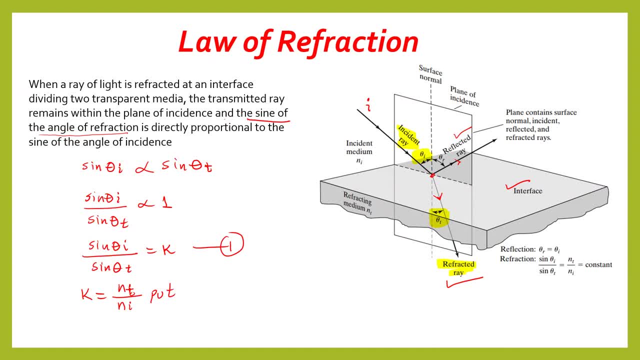 in which you have, in which the ray is being transmitted, that is, you have index of refraction n. you can say that is index of refraction, n is index of refraction and n is basically. 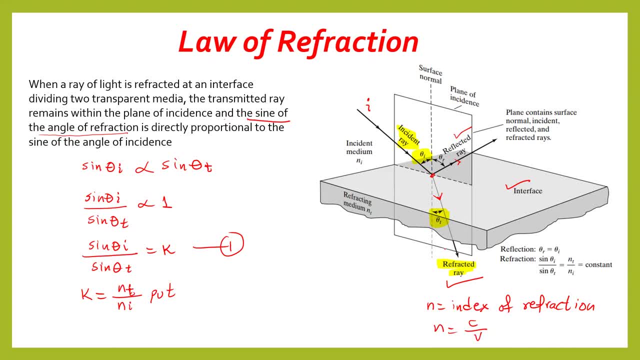 the ratio speed of light divided by speed of light in that medium okay, its value is approximately for air 1.04, and for glass 1.4,. these are the values. speed of light.